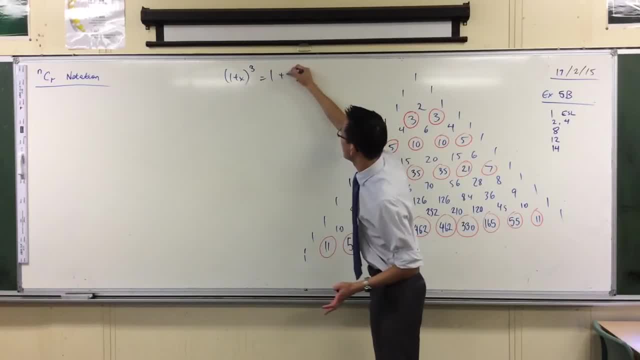 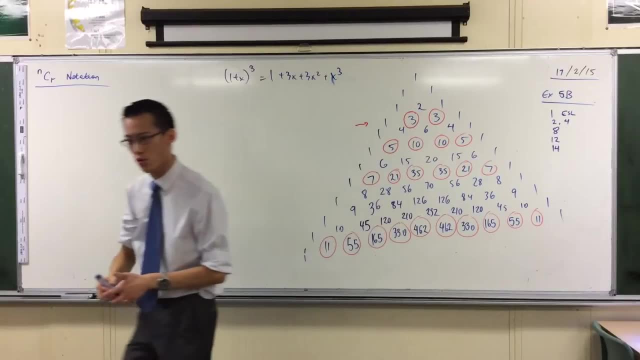 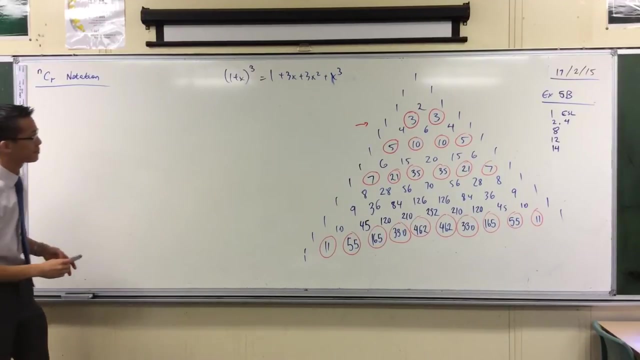 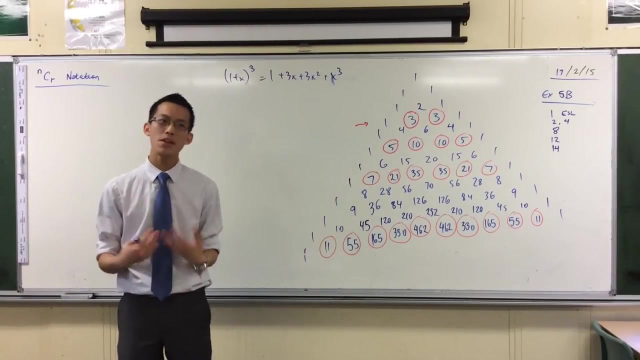 So we can expand these things, and when we do that, we find that these numbers from Pascal's triangle mysteriously appear. So that's why this has appeared right, But clearly there's some structure going on here and we want to be able to talk about it. 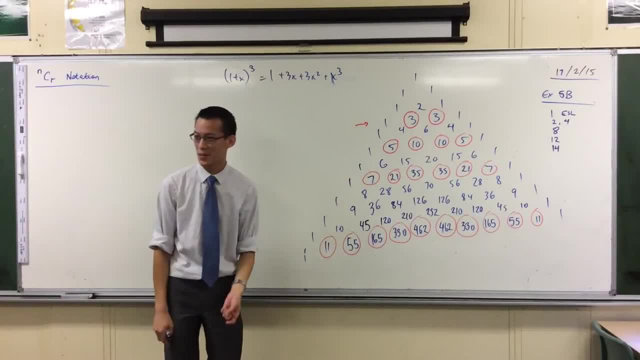 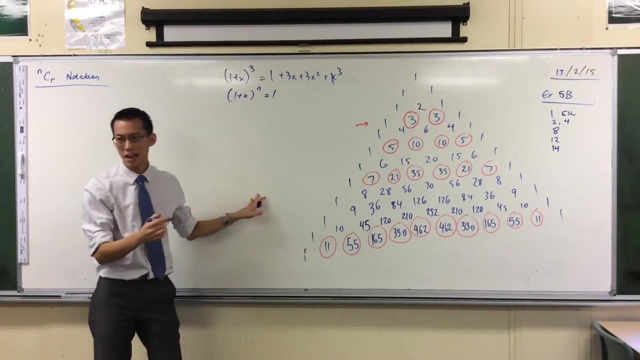 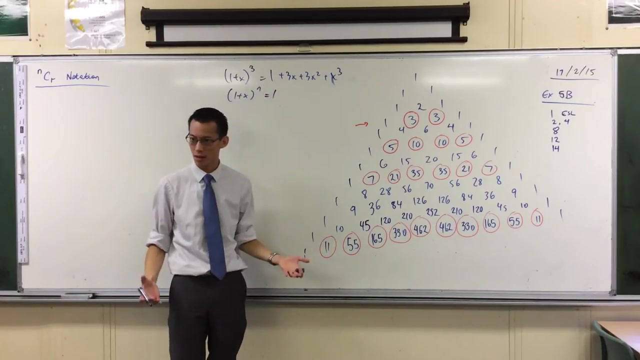 Number one without having to draw out Pascal's triangle every time, and number two in general terms, right Now. that's harder to wrap your head around. This is harder to conceptualize than this, right, Because I can write down the first number. but after I've written down my first number, I don't know what to write, because I don't know what n is, so I don't know what row I'm in, so I'm stuck. okay, 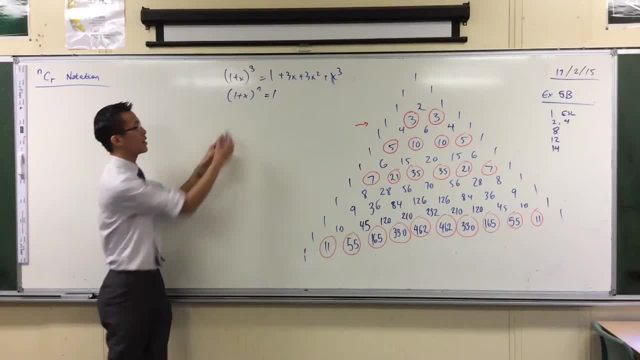 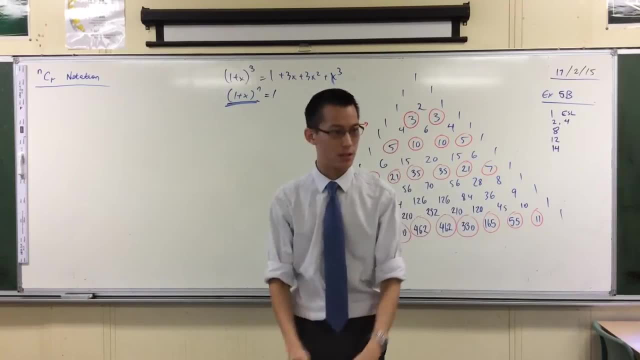 So I'm going to introduce some language, some notation which will allow me to. I'm going to dig at this without even knowing what n is. okay, So let me introduce this to you, let me define it for you. okay, Write this down with me. 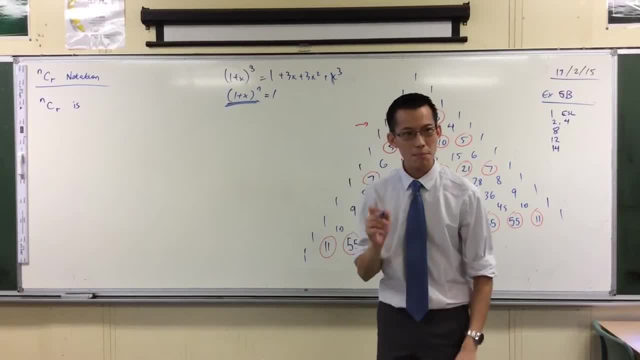 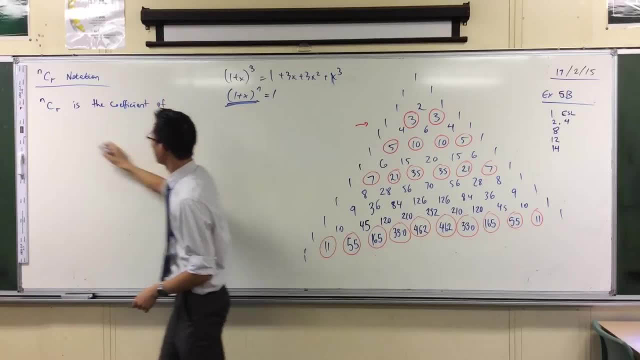 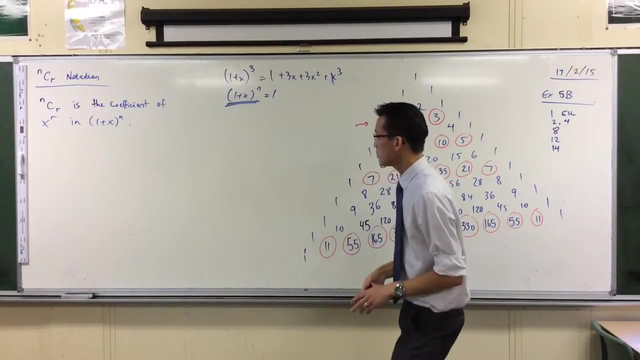 ncr is. ncr is a number, okay, In particular it's the coefficient of x to the power of r in this precise binomial. okay, I should say in the expansion of that binomial. but that's kind of implied. 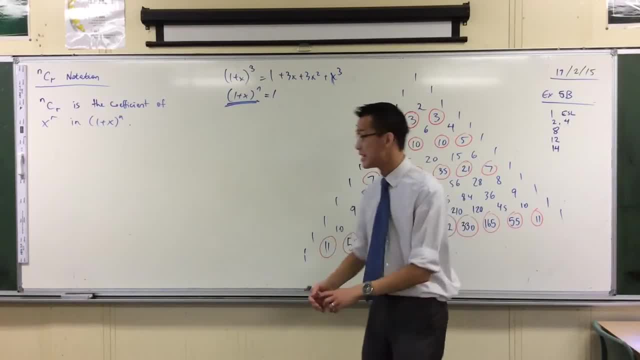 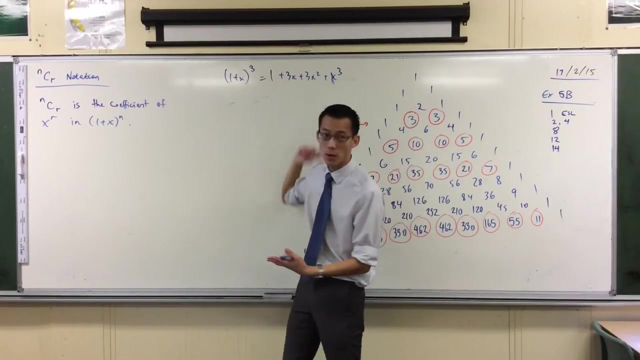 Isn't it Right? So let me give you a nice easy example stemming from this guy. okay, I'm going to write this up. We have all of the coefficients- 1,, 2,, 3,, 4, and now I can write them without knowing what they're actually equal to. 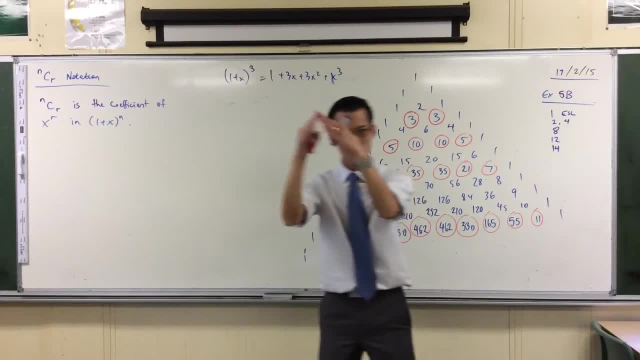 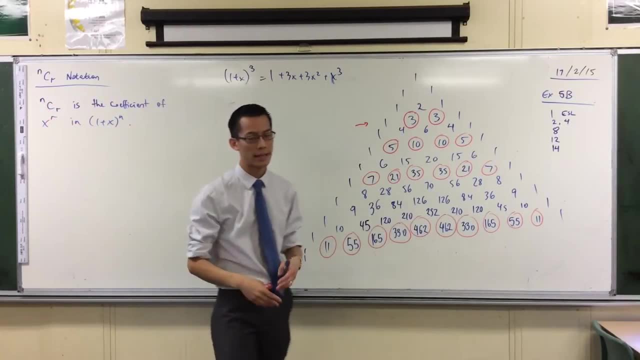 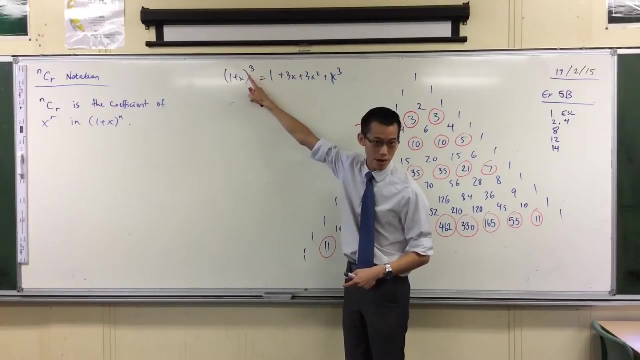 using this notation. Okay, now pay attention. ncr- right, And I do write it with that funny superscript, normal subscript format. okay, ncr- the n refers to the power that I have. okay, So in this case it's 3.. 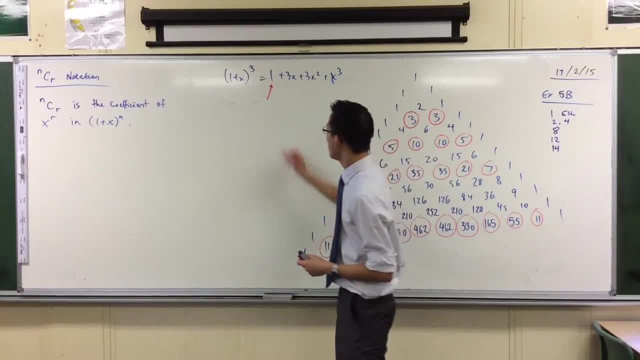 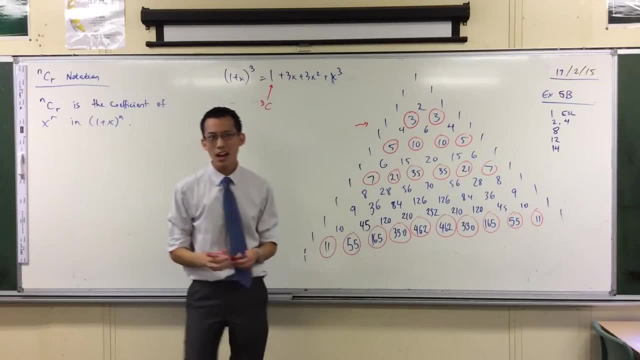 So let's have a look at this one, this first coefficient. right, It's going to be 3c. Now, what will be this number down in the bottom corner, this r number? Now, it's kind of hiding there, isn't it? 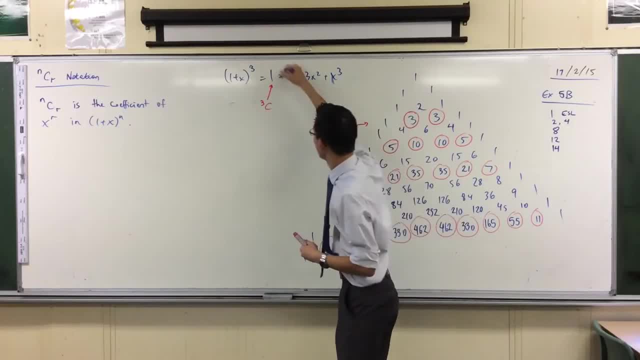 It's the power of x that I've got, but in this case the power of x is 0, isn't it See why mathematicians often start at 0? It's not just arbitrary, It actually makes sense in this context. 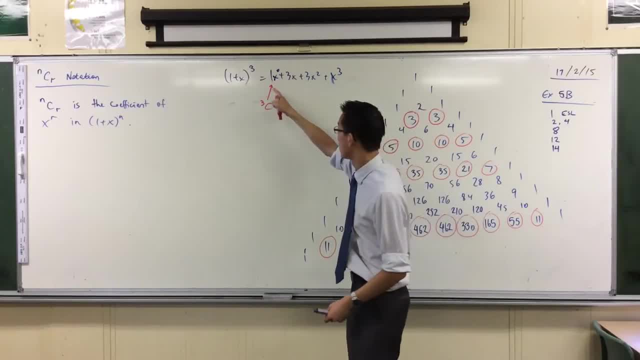 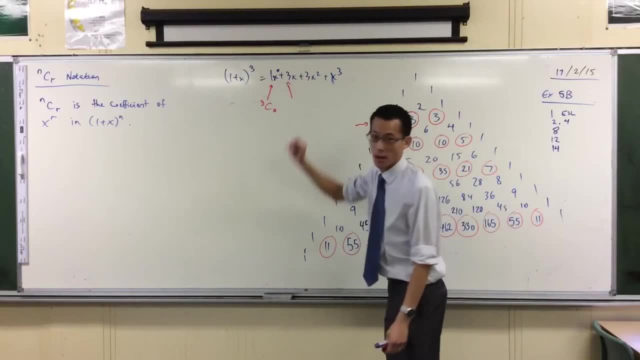 Okay, so that that first number there, namely 1, right, That's 3c 0.. That's the definition of 3c 0.. This next number along right, It's ncr. so the n is still that power. it still stays the same. 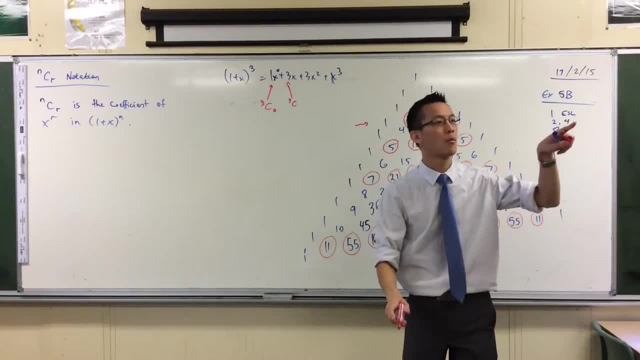 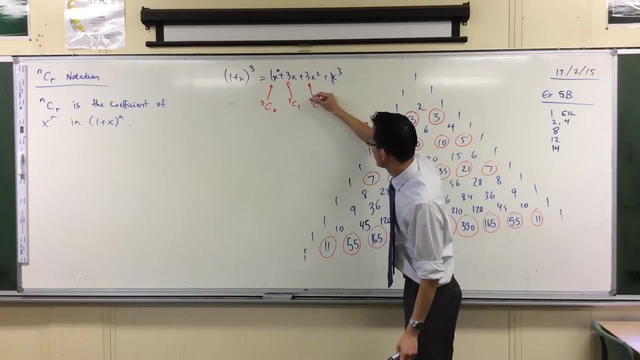 It's going to be 3c, but the power has moved up, one hasn't it. Okay, so this is 3c 1. And now you can just kind of unfold the pattern from there. You've got 3c 2 there. 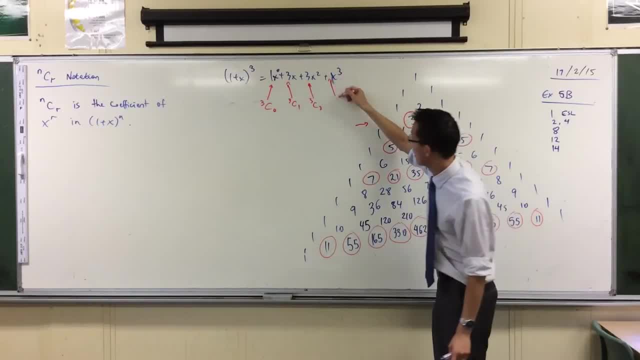 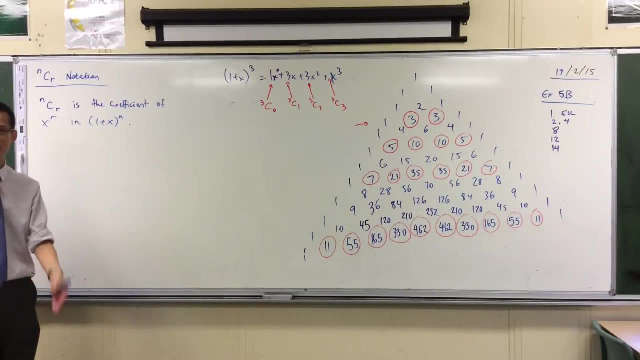 and hiding in there that 1 in front of the x cubed. That's going to be 3c 3.. Now I'm just going to pause for a second, just to caution you, because I know in this class there are going to be a significant enough number of you. 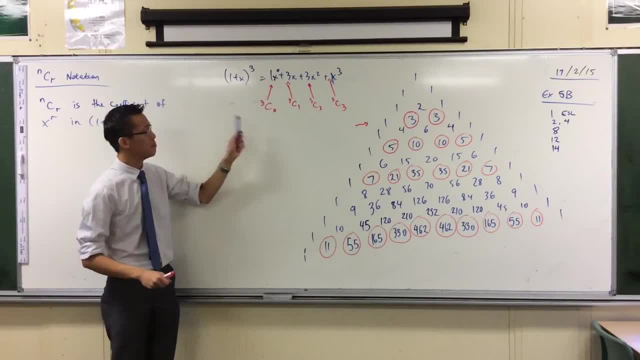 that you recognize that this. this means more than just what I'm defining it to be. It has a much broader meaning than what I'm starting with. okay, But I want us to start here and we'll get there in time, and it will be confusing if we introduce it all at once before you understand how the pieces fit together. 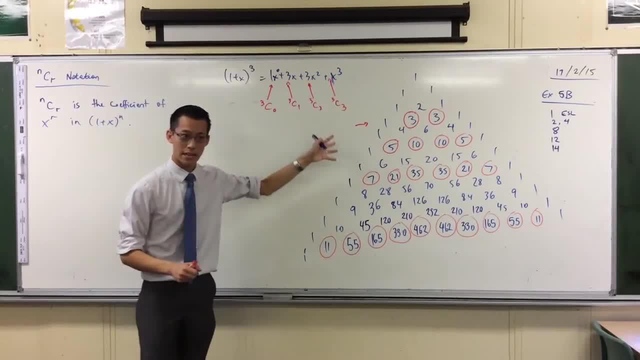 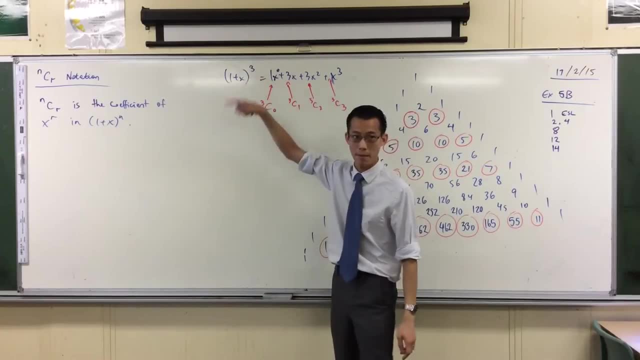 Okay. So if this is a particular, particular example, remember one of the reasons why I was pulling out introducing this whole language is so I can start to generalize and not just think about what it's to the third power or the fourth power. 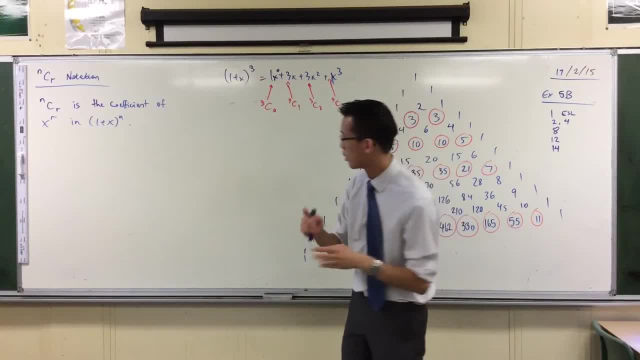 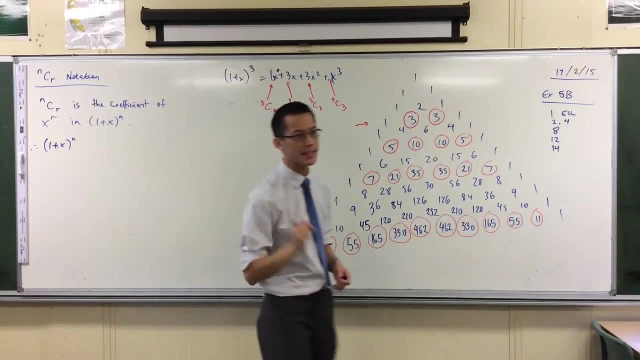 or the fifth power, but to any power, right? So let's write this out: What is 1 plus x to the power of n in this scheme? How would I write it? Okay, well, because it's starting with a 1, right? I could say it's always going to be 1.. 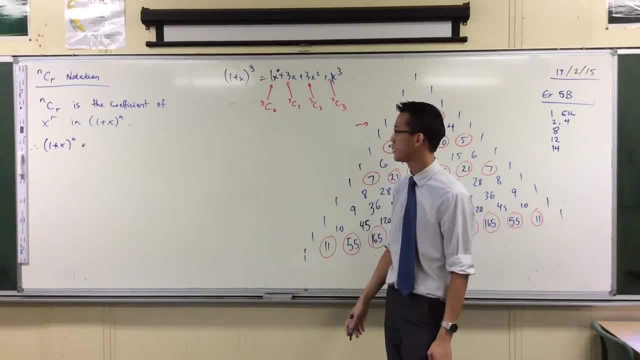 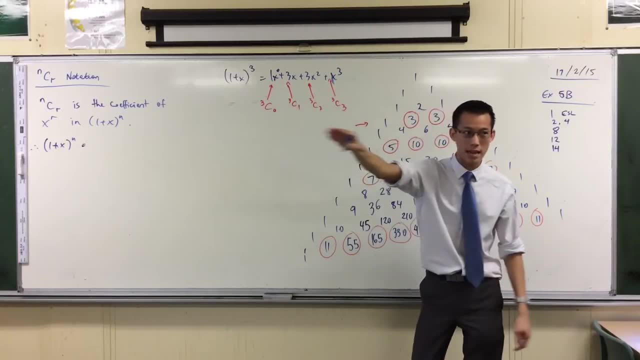 No matter what n I have, the first time will always be 1.. But I can write it in a more helpful descriptive way: right, See how? the number at the top, the n, that's staying the same the whole way through and it relates to the power. 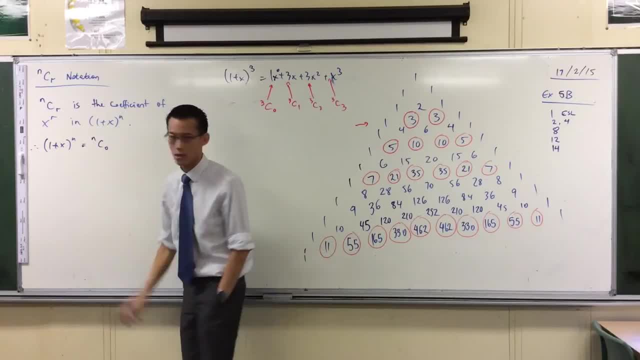 So the first term should be nc0, right? So that top term is going to stay put, If you want to think about it this way, it's up the top, just the same way, the power is up the top, so you can sort of match them together. 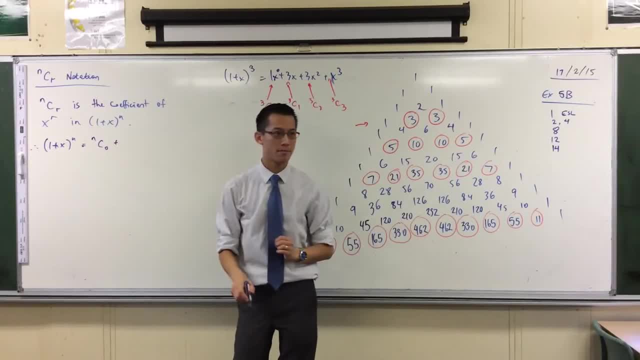 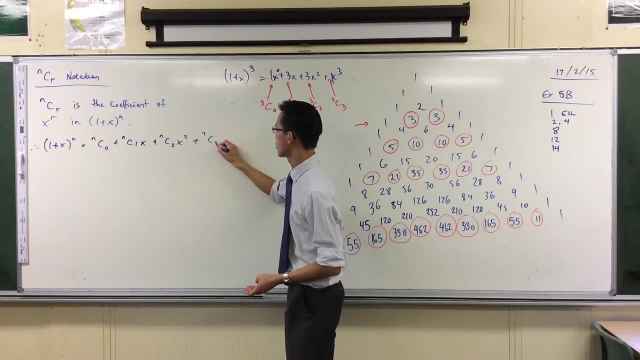 There's the first term, Now the next term, the n stays the same, but I'm moving up 1 by the power right, Which of course means there must be an x term that comes with it, right. And now my pattern continues. I'm going to have x squared, I guess I'd have x cubed, and so on. okay, 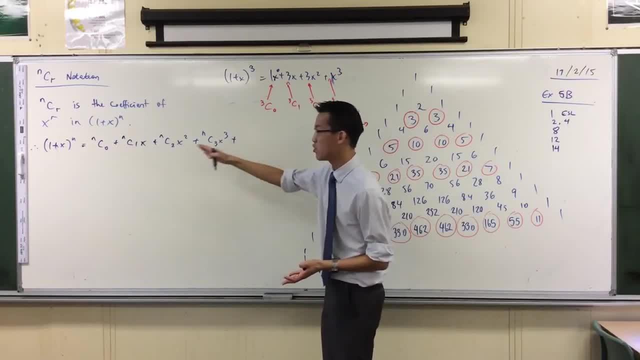 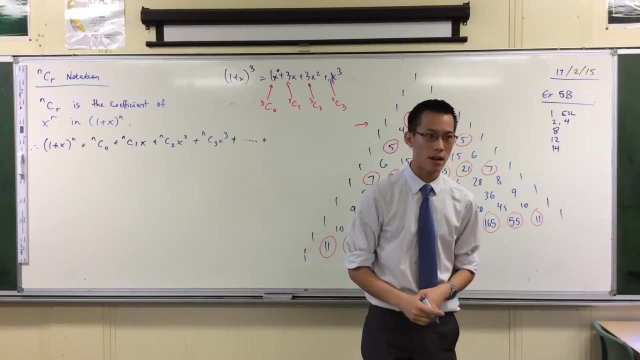 Now I don't know what n is right, So this series of terms is going to go for some undetermined amount of time, but it does end. It's not infinite, right? What would be the very last term on the end, okay? 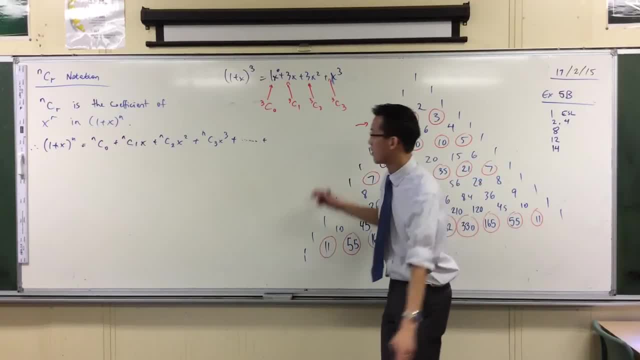 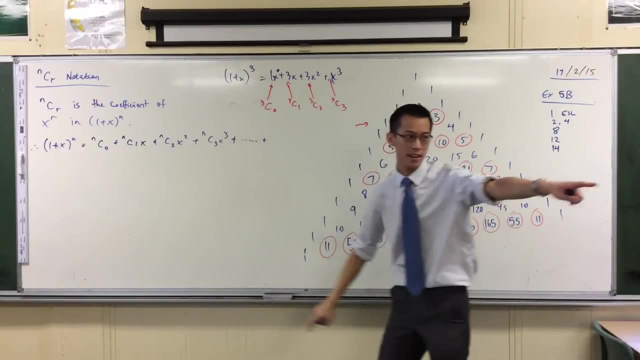 nc0.. So, yeah, yeah, let me see. okay, First, my x will be just like here: This power is going to match what you started with right, And then, secondly- I think, Doris, you said it- 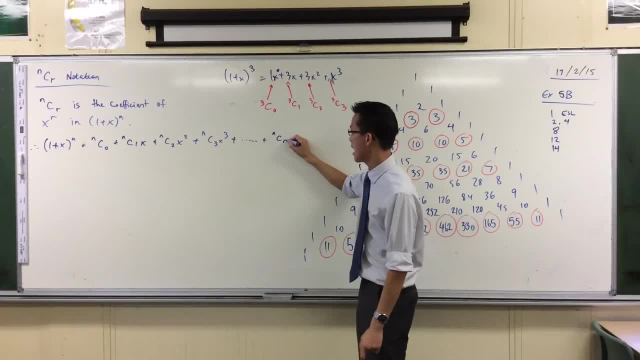 the coefficient is going to be ncm. Okay, so that all matches up right. So far, so good. Does that make sense? Okay Now, just before I go into this and introduce sigma notation on your calculator, which you should get out now, 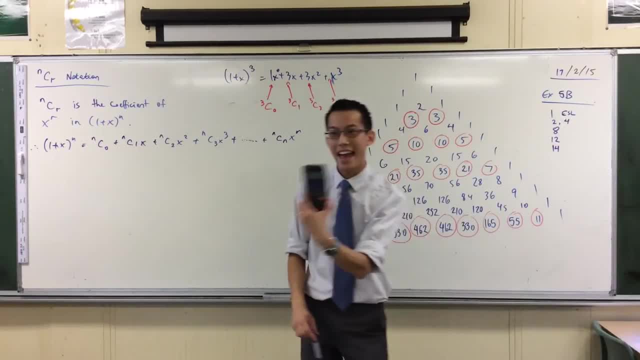 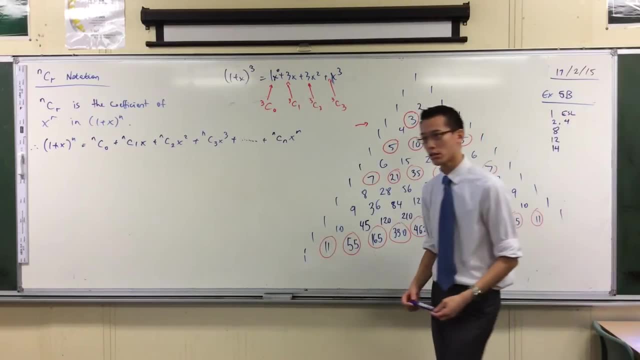 ncr notation. it's all right, you can see it on the screen. ncr notation is on your calculator. You might not have noticed it If you go down to your big buttons there right and if you look on top of the multiplication and division signs. 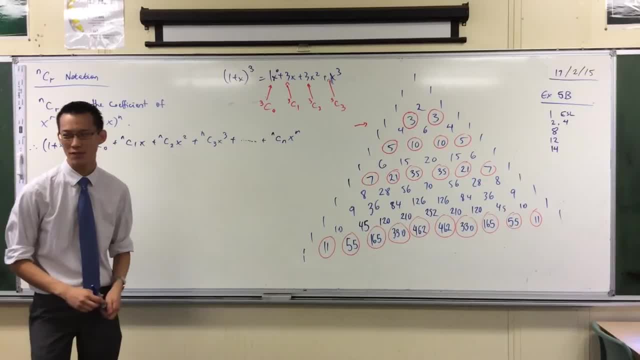 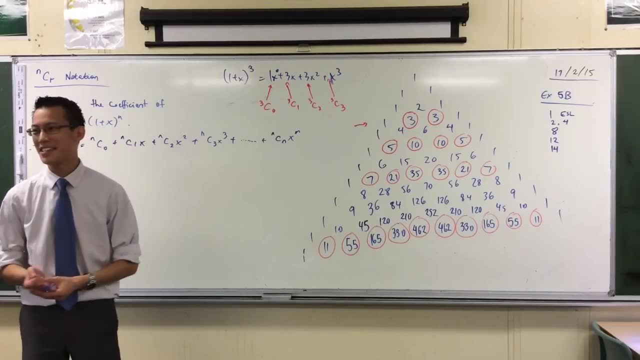 you see these operations hanging out there which you've never really paid attention to, right You'll notice there's an npr which has nothing to do with National Public Radio in the US and there's an ncr which clearly, by the way they're set out, have something to do with each other. 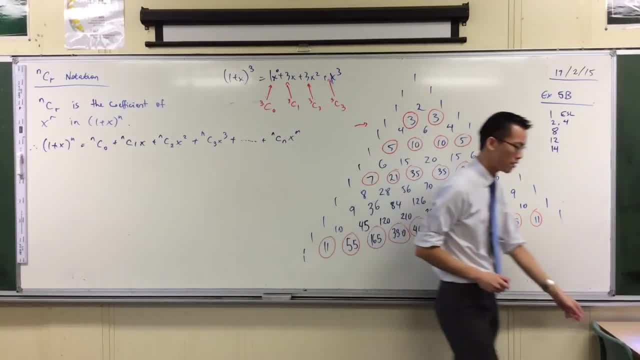 but we'll dig into that in a few minutes. Okay, ncr is the one I'm interested in. So, for instance, let's have a look at this guy: 3C0.. I punch that in in my calculator by saying: 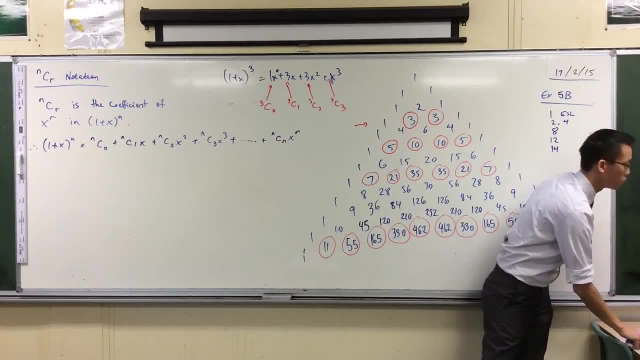 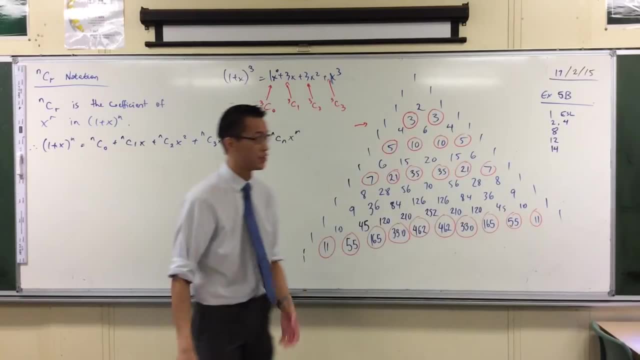 3, you're going to have to go shift. whoop, let's turn it on, that'll help. 3, shift 0.. So you get that funny looking C right, which is its way of indicating this right. 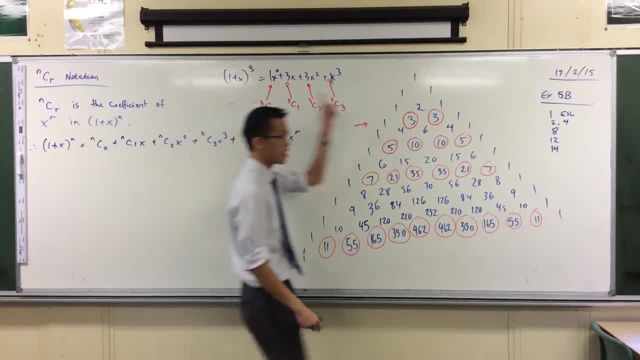 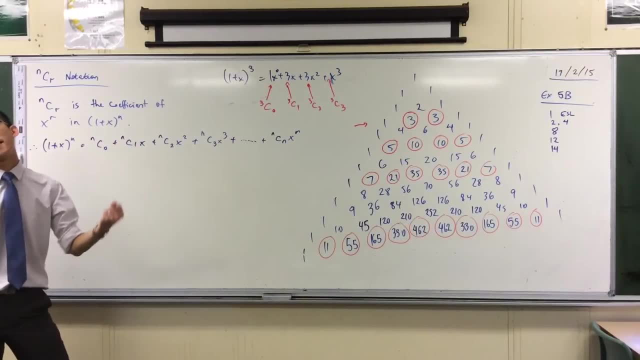 So I've literally written it: 3C0, okay. And, as we expect, when you hit equals, you get 1, okay. So for those of you who don't know, for those of you who are kind of like, 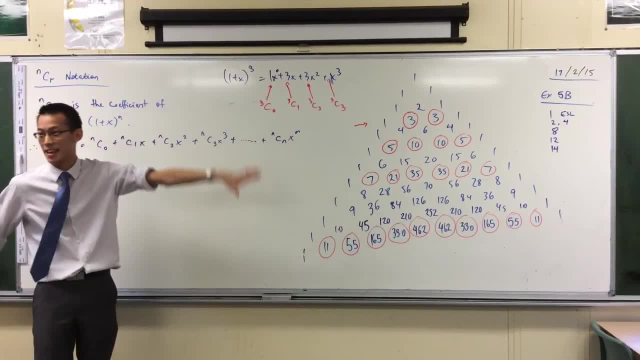 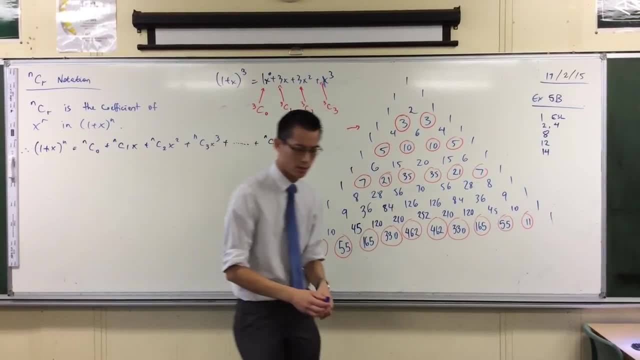 oh man, I have to keep flicking back to where I've drawn Pascal's triangle. I have to keep looking at this thing, right, Remembering that these coefficients match up exactly to these numbers, right, For instance? let's just do a quick experiment. 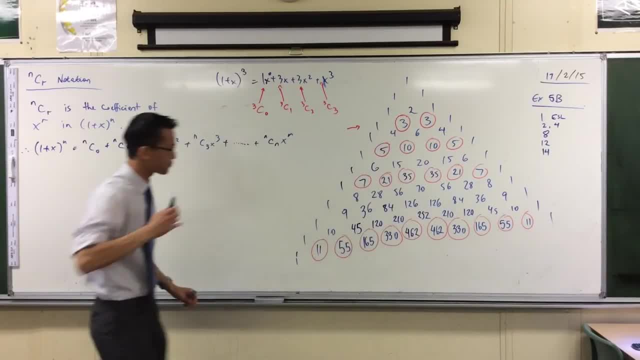 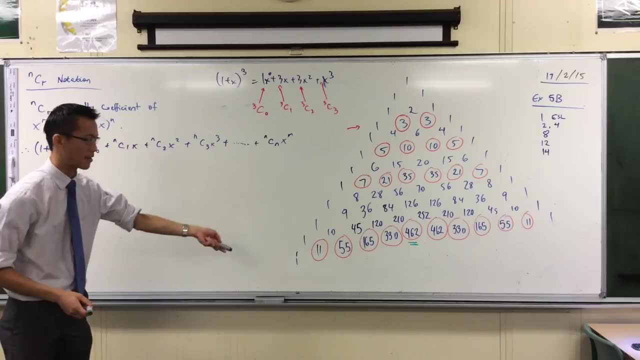 How would you work out a term like: okay, so 462.. That's the biggest number in my Pascal's triangle that I've drawn out. okay, What ncr does it correspond to? Now do it slowly with me. What's the n stand for? 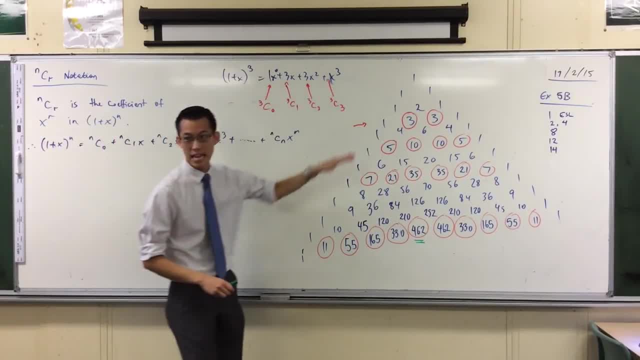 It stands for power right, Which in Pascal's triangle, means it stands for row right. That's the power that I'm interested in. is the row that I'm looking at? okay, So this is the 11th row. Does that make sense? 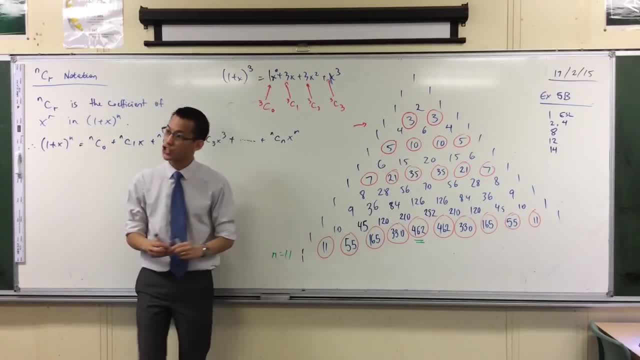 So I've got n equals 11 here. Now which term am I actually interested in? right, There's two ways you can think about this. Firstly, I can just count them up, can't I? So I've got term 0, 0.. 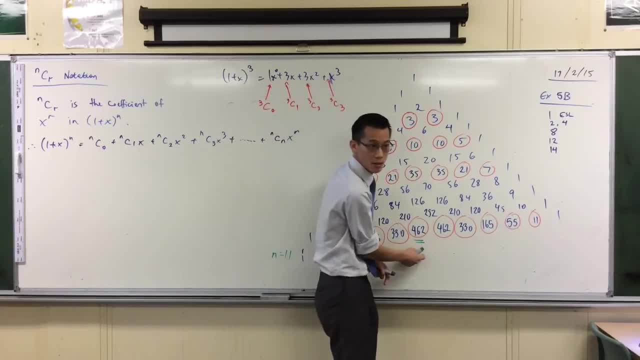 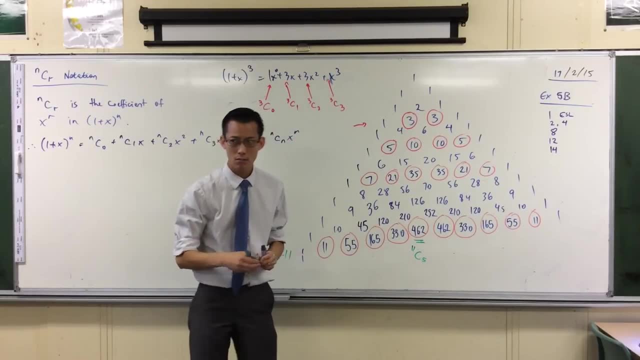 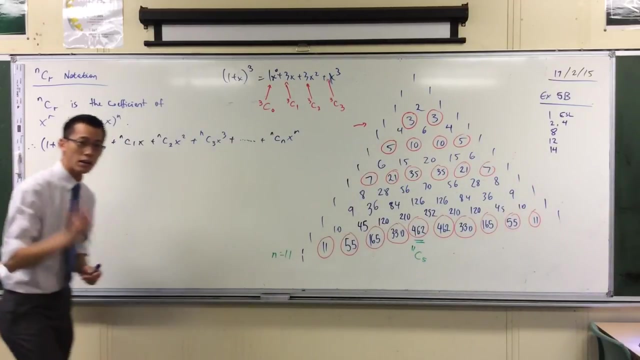 1, 2,, 3, 4, 5.. I've termed 5 there, right? So this should be. it should be 11c5, right? Let's check it. Sure enough, okay, That was the first way. 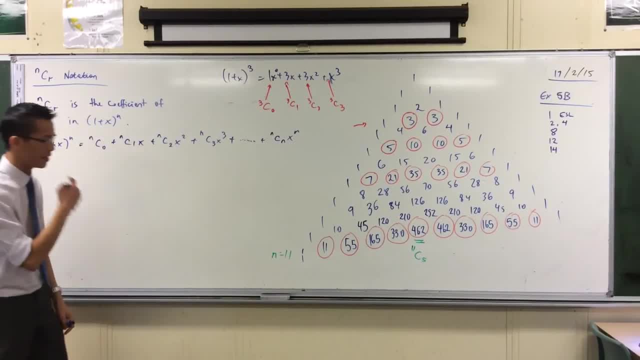 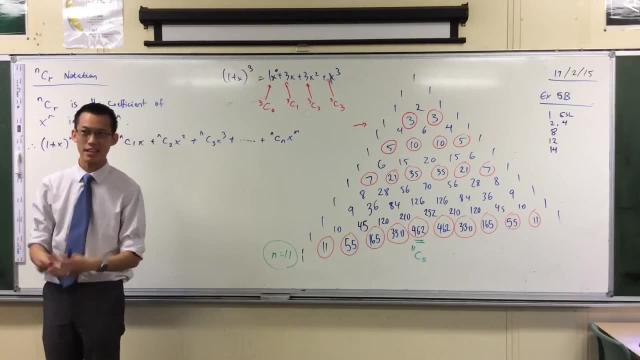 You could have just counted it out. There's another way of thinking about it. Before drawing any of this, if I tell you a row of Pascal's triangle, you ought to be fairly easily able to tell me how many terms there will be in that row. 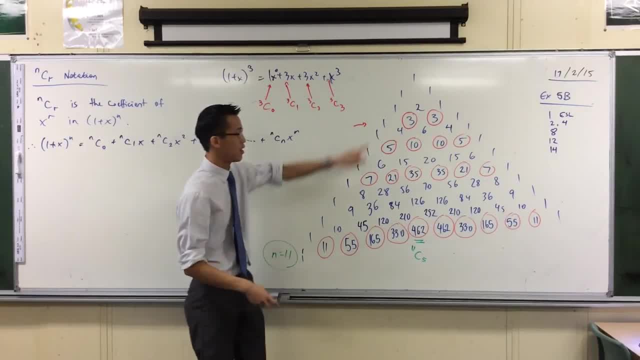 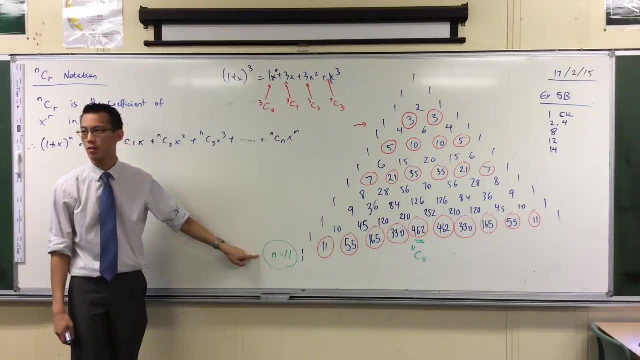 Because they keep getting bigger, don't they? For instance, the third row has 4 terms. The seventh row has 8 terms, So the 11th row is going to be 12 terms. right Now, if there are 12 terms, watch out. 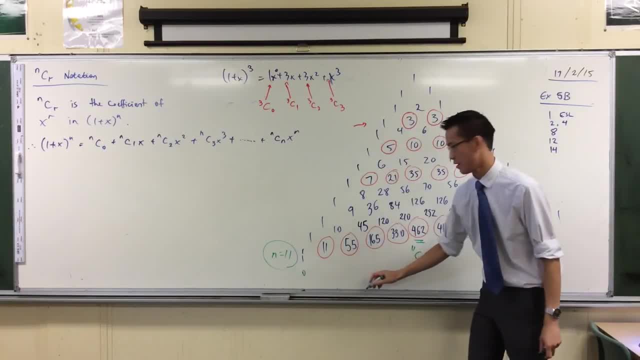 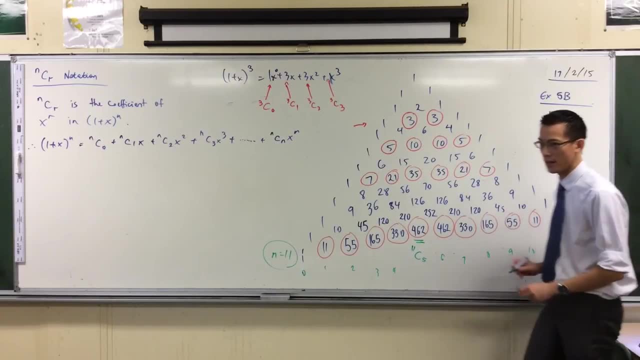 I start from 0.. 0. And then 1,, 2,, 3,, 4,, 5.. 6,, 7,, 8,, 9,, 10,, 11.. Now the question I posed at the beginning was: 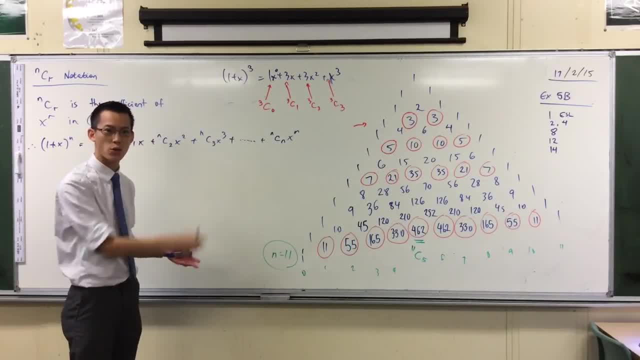 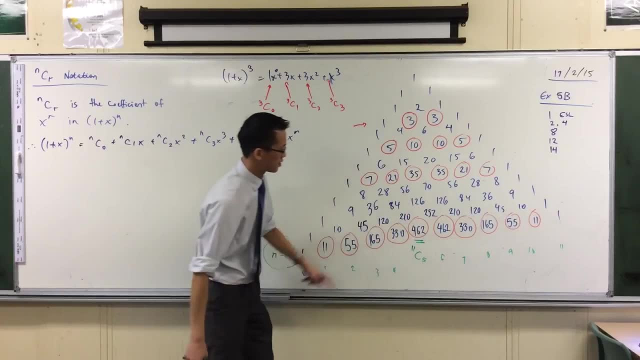 I wanted the biggest term there. The biggest term in any row of Pascal's triangle will always be the middle one, right In the middle, because there's symmetry to it. yeah, So some of them have one middle term. Why does this one only have one middle term? 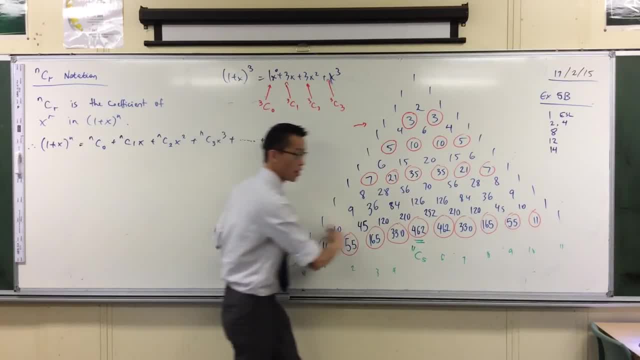 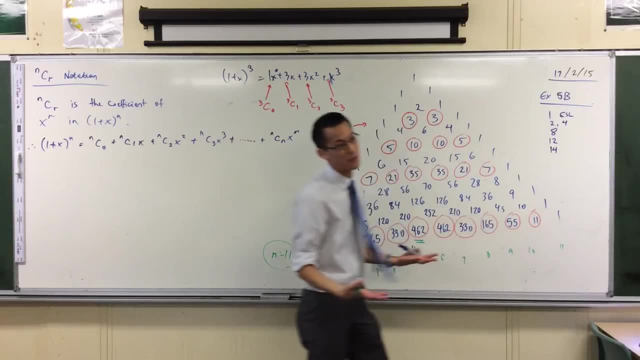 Because it's got an odd number of terms, right? So there's 1.. It depends on if you're thinking about n or the actual number of terms, right? So this is the nth row with n plus 1 terms. So in this case you can see. 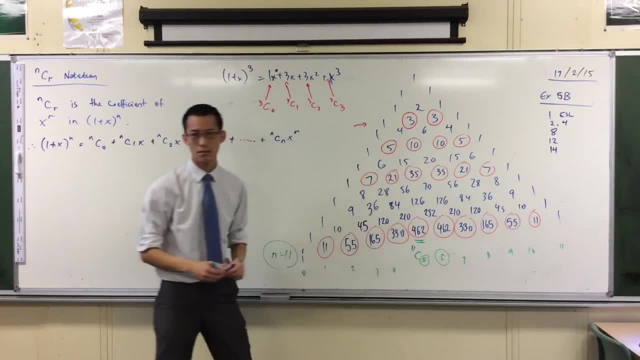 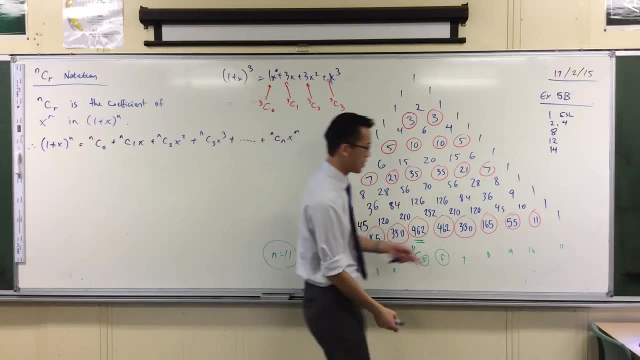 it's going to be terms 5 and 6, right. The way that I would think about that, I guess is the way I get middle- is by divining by 2, right. So that would be 11 divided by 2,. 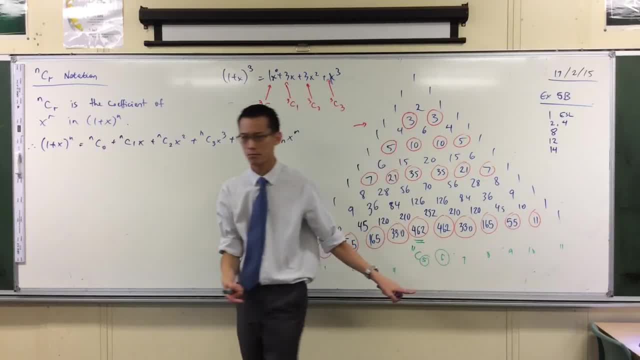 which is 5 and a half, which tells me either of these would be fine. Does that make sense? Okay? 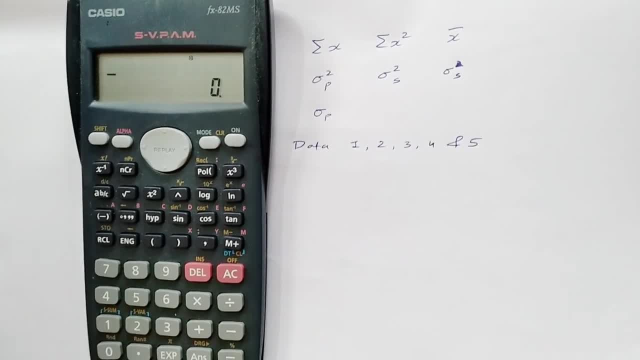 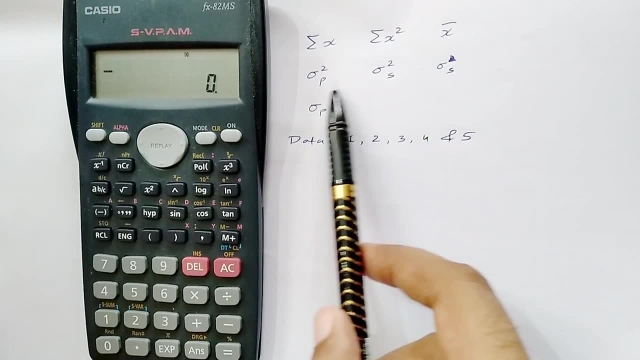 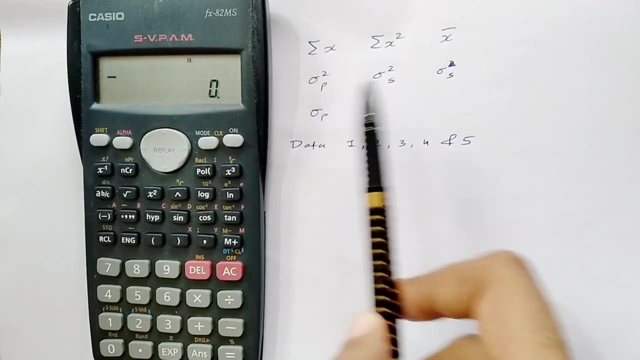 Namaste friends, In this video I am going to show you how to calculate sum of the values, sum of square mean, variance of population, variance of sample, standard deviation of sample and standard deviation of population for a given data. We have taken a simple data: 1,, 2,, 3,, 4 and 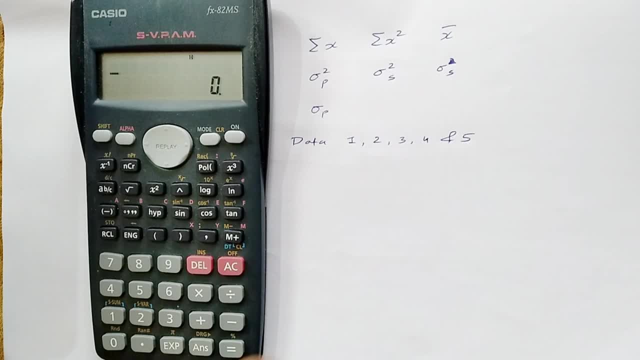 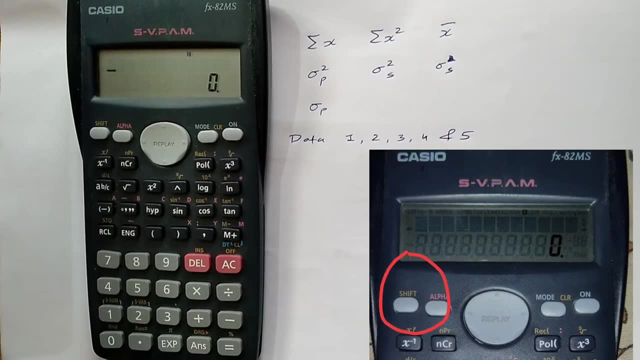 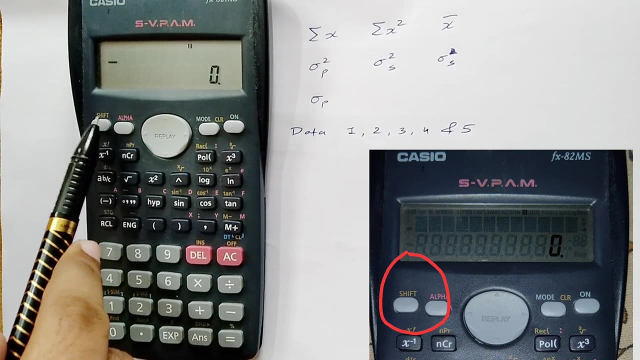 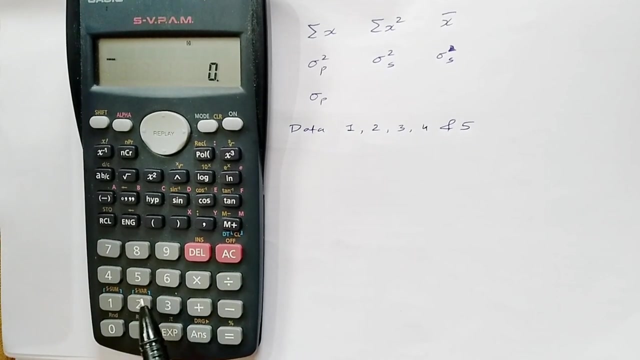 5 and we would be using this calculator. So before we switch to calculation part, I would like to show you this shift key. So the shift key here the shift is written in the yellow. So when we press the shift key, all the symbols that are in yellow that got activated. 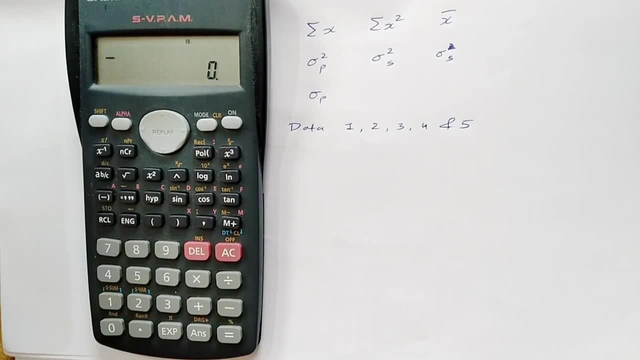 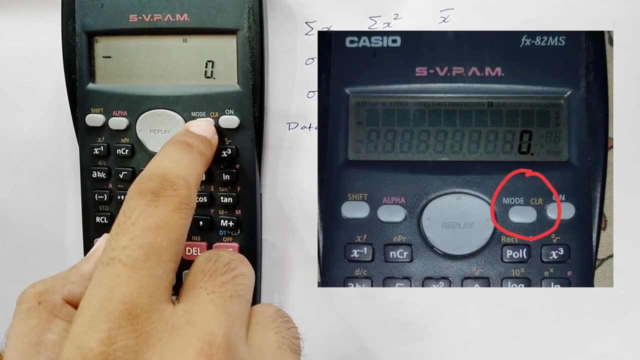 So when we press the shift key, all the symbols that are in yellow that got activated. So now let's first do our first step. The first step would be press shift, then yellow gets activated. So yellow here is CLR. that means clear, So clear. We want to clear everything. 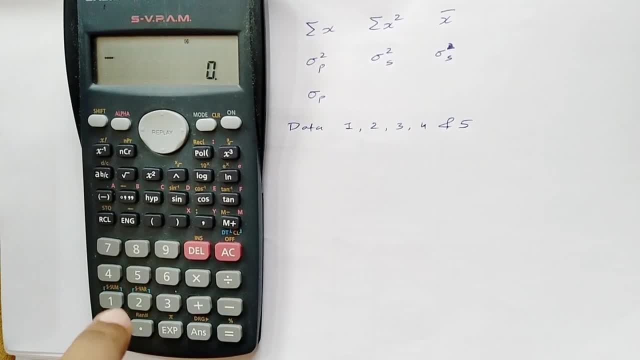 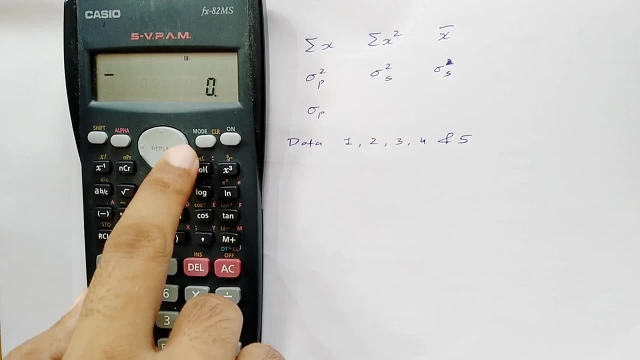 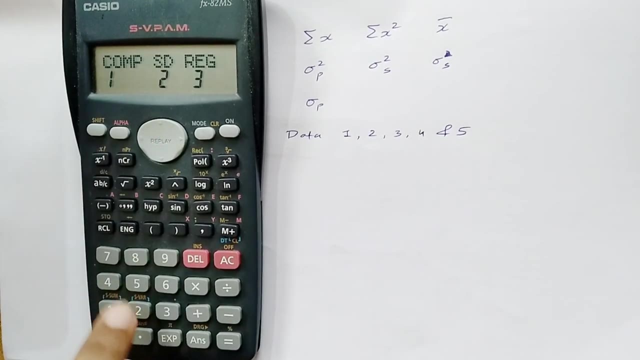 So 3 equal to equal to What this will do. This will delete all the previous data that is present in the system. Okay, Now press on the mode. Then we want this SD. So the symbol is 2.. So we will press 2 here and then we will start. 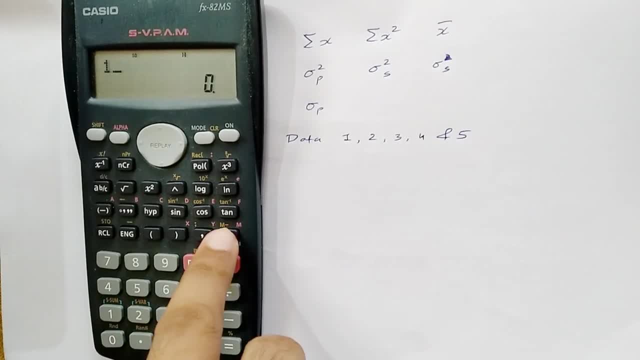 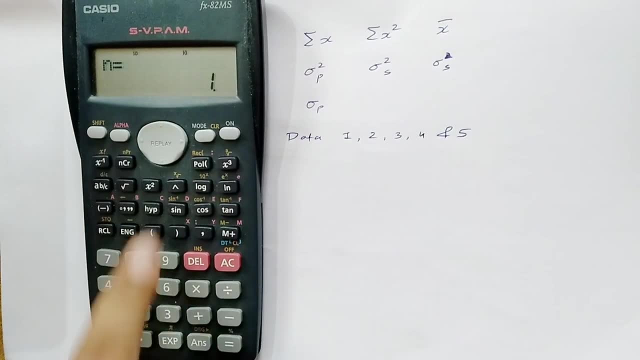 entering the data. So first value, that is 1.. M plus this will add the data into the system. So N equal to 1.. That is our first observation is 1.. Now we input our second data, that is 2,.